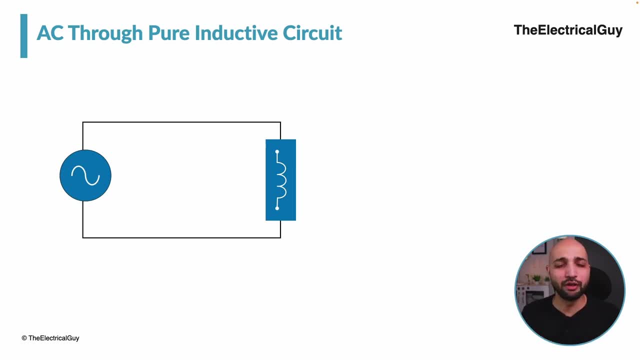 considering the inductor is pure. Now, in the previous video we discussed about AC through a resistive circuit and we saw that resistance simply opposes the flow of electrons, So it really doesn't matter if it is alternating or a direct current, or you know, 5 ampere, 15 ampere, 500. 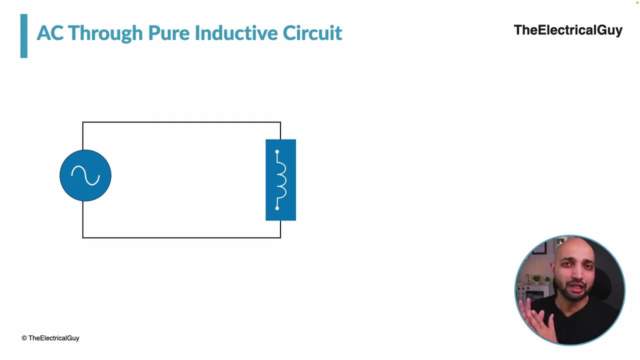 ampere, it really doesn't matter. Resistor simply opposes the flow of electron. But when we talk about an inductor, Inductor does not behave same to that of a resistor. What inductor does is: inductor opposes the change in current right. and how they oppose? they oppose the change in current by drawing or 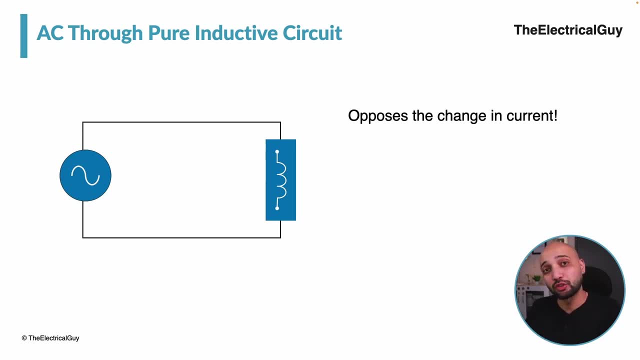 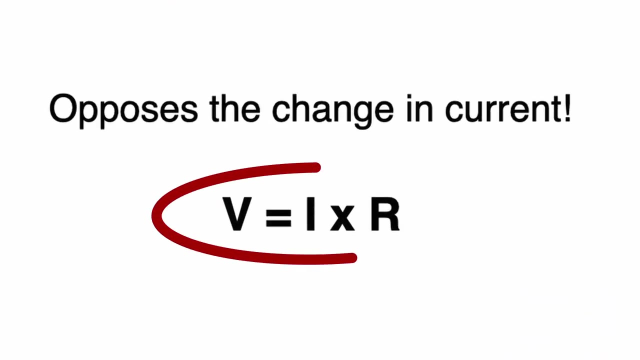 supplying the voltage which is, you know, directly proportional to the rate of change of current. So inductor tries to maintain a constant current that is flowing through them. and how one can control current? well, that takes us back to the ohm's law, which says voltage is directly proportional to the current, provided the resistance is constant, right. So if 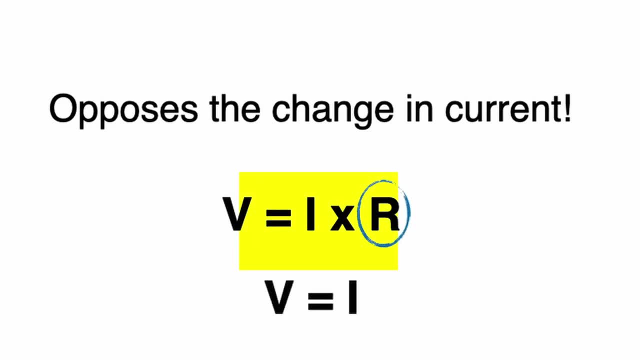 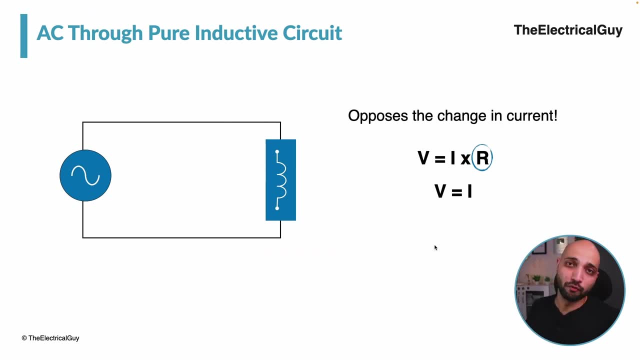 resistance is constant, then it is very much clear that the current is directly proportional to the voltage. One can control current if he or she can control the voltage clear. and the same thing happens in case of inductor. Now, as we have seen, inductor opposes the change in current. So if 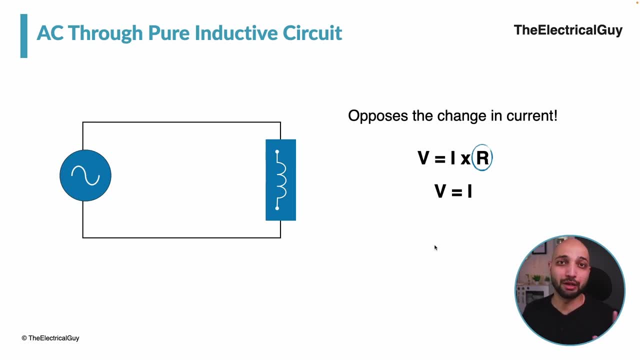 you are passing a continuous current through it, it is okay. But if you are passing an alternative current, then the inductor is not okay. Inductor will start opposing that and how it oppose. So let's say, current is going from zero to its maximum position. 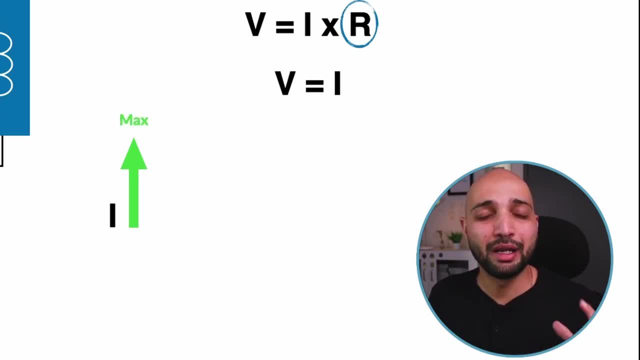 Now what inductor does is: inductor tries to maintain the current at a constant level, and to do that it drops the voltage to zero, so that it can bring back the current, you know, to its previous position, that is the zero position. right here It drops the voltage to zero, So, similarly, 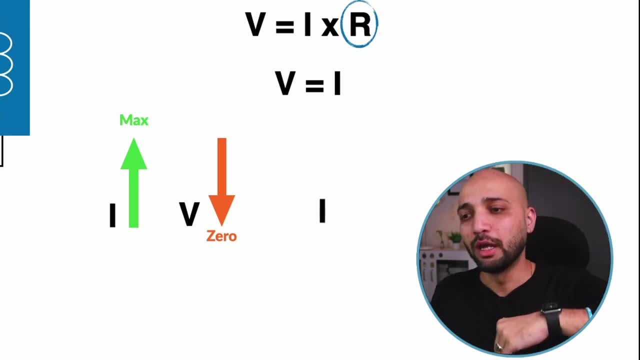 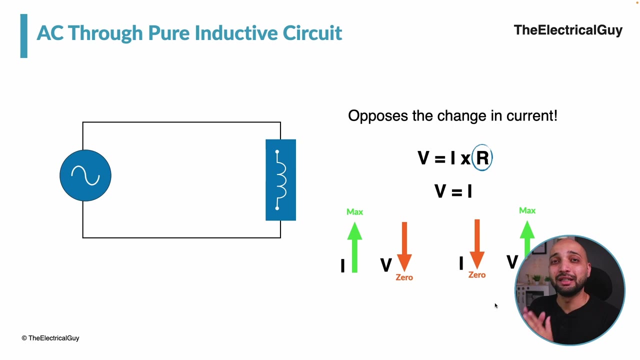 when current goes down from maximum to zero, what inductor does is inductor push more voltage in the circuit so that the current can get back to its original position. that is the maximum position, right, clear, And that is the reason why you will see in an inductive circuit, whenever current is. 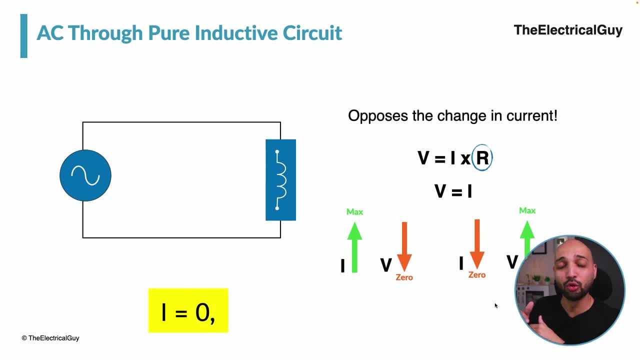 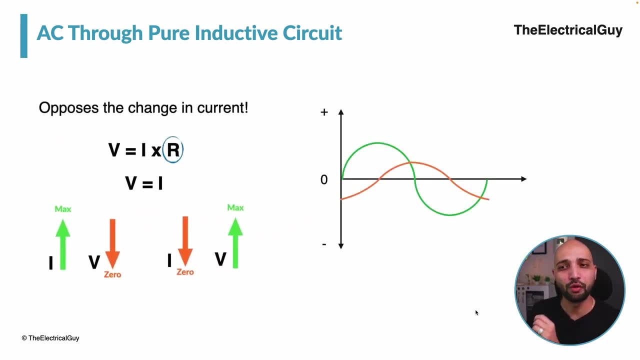 maximum, the voltage is zero, and when current is zero, the voltage is maximum. Now, with this understanding, we can actually draw the wave form For voltage and current in an inductive circuit. So on the right hand side you can see the green waveform indicates the current waveform and the orange waveform indicates the voltage waveform. 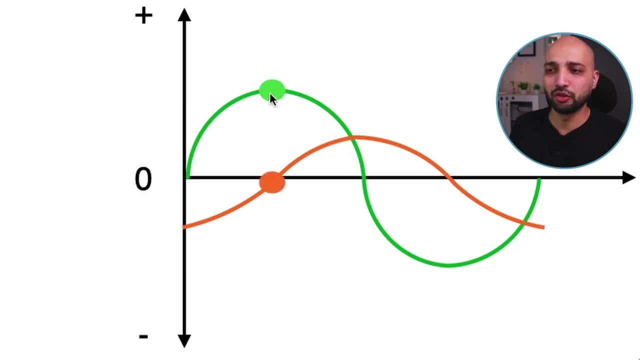 So you can notice, when current is maximum at this position here, the voltage is zero. Why? because the inductor is trying to drop the voltage so that the current will also drop, which was its original position, that is zero. Now the next step. you see, when current is zero, the 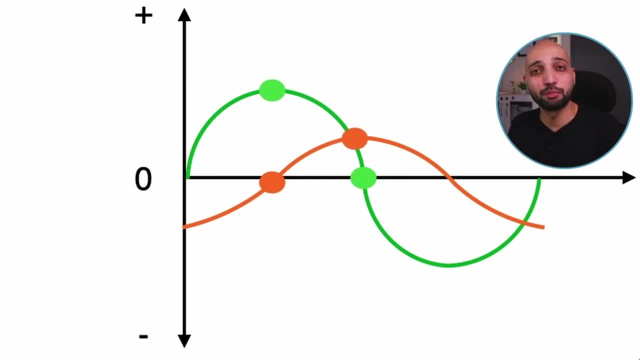 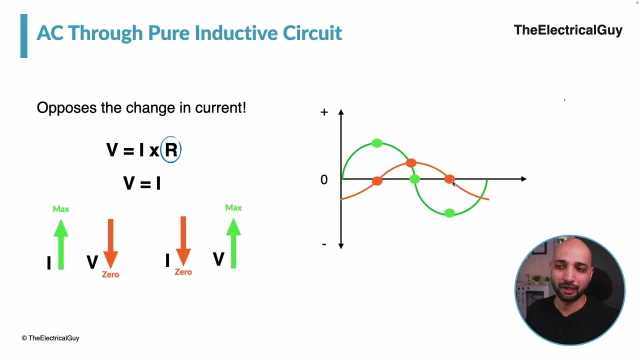 voltage is maximum. Why? because again, inductor is pushing more voltage so that the current will get back to its previous position, which was the maximum position. So, similarly, when current drops to its negative peak, the inductor drops the voltage to zero right, and that is the reason why. 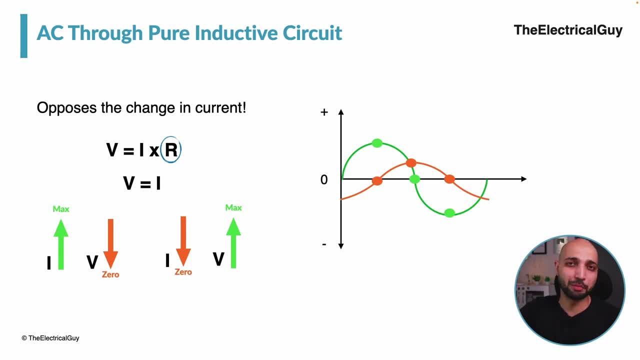 there is a difference between when the current reaches to its peak value and when voltage reaches to its peak value. And if you notice that if, let's say, current is reaching to its maximum value at 90 degree, then voltage is reaching its maximum value at 180 degree, So there is a gap of 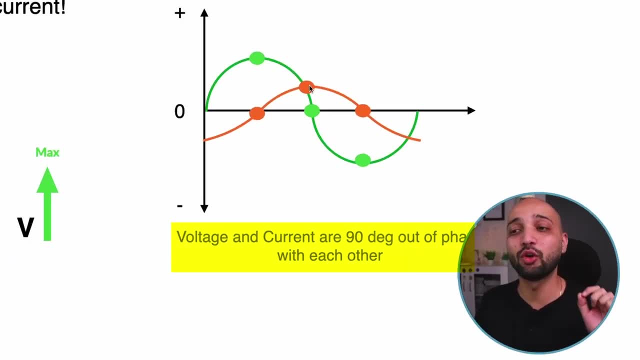 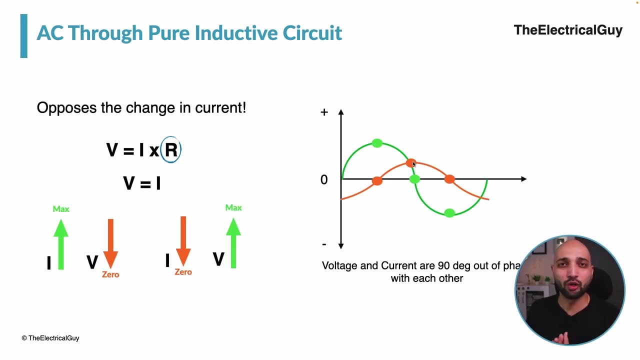 90 degree right and hence in inductive circuit, voltage and current are said to be 90 degree out of phase with each other. Clear, So that is how voltage and current behave in case of purely inductive circuit. They are out of phase by 90 degree with each other. Now the 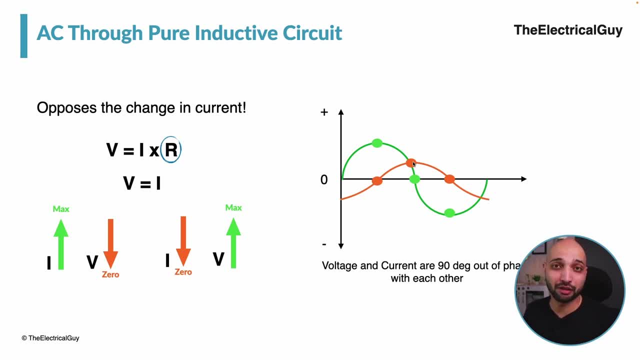 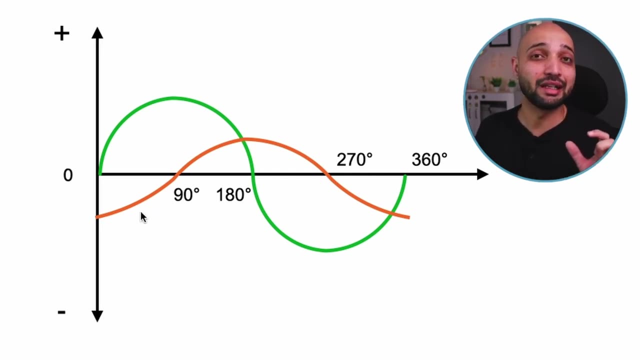 interesting part. Now we are going to discuss about the power situation in an inductive circuit. So let us consider the first section here, wherein you have to focus on 0 to 90 degree Now. in this portion you will notice current is positive but the voltage is negative, and power is what power? 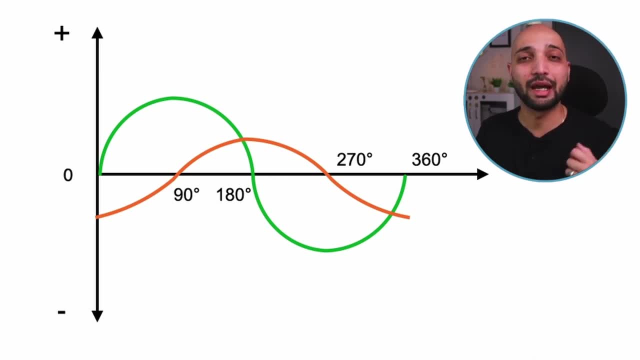 is multiplication of voltage and current. So when you multiply a positive value with a negative value, the resultant is always a negative right and, as a result, the power during this portion is also negative. right Now let us focus on 90 degree to 180 degree Now. during this portion, both voltage and current are. 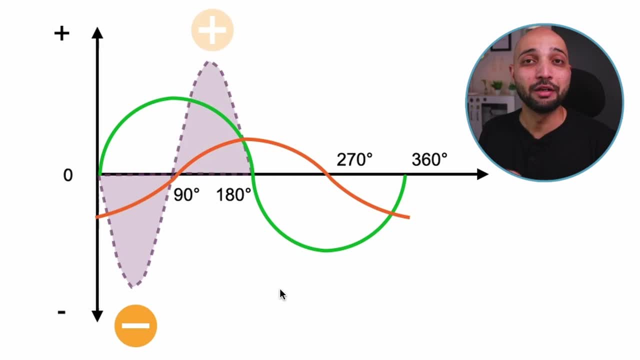 positive. So definitely the output power will also be positive. Clear In the third section: 180 degree to 270 degree, the current is negative but the voltage is positive, but still the resultant will be a negative power. And during 270 to 360 degrees both voltage and current are negative. 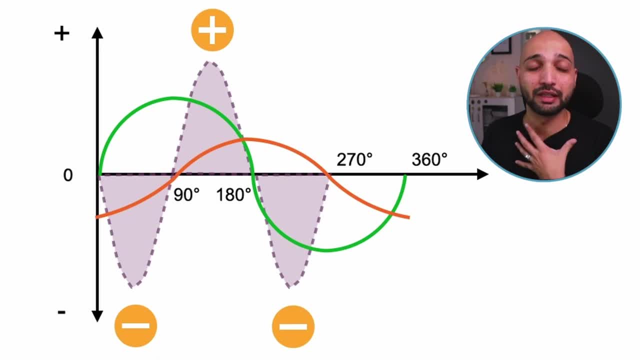 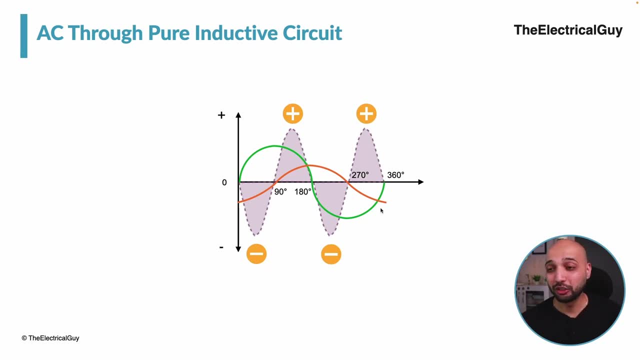 and negative multiplied by negative will always give us a positive output, and hence the power will also be positive. Now, the interesting fact about this type of power is that you will notice we have two equal positive peaks here and two equal negative peaks, and they cancel out each. 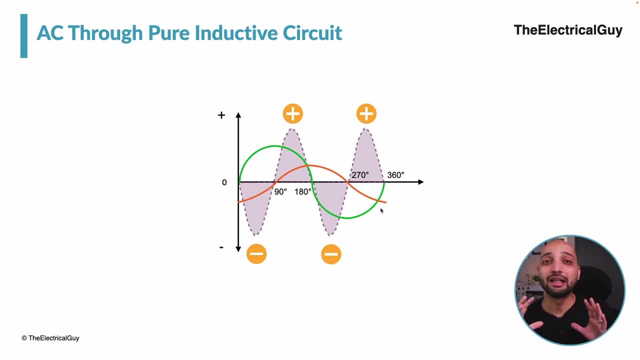 other because they are equal and, as a result, the actual power consumed by an inductor is 0. right, it is zero. Now us understand what is this negative power mean? well, negative power means inductor is actually delivering power back in the circuit, and the positive power indicates that inductor is. 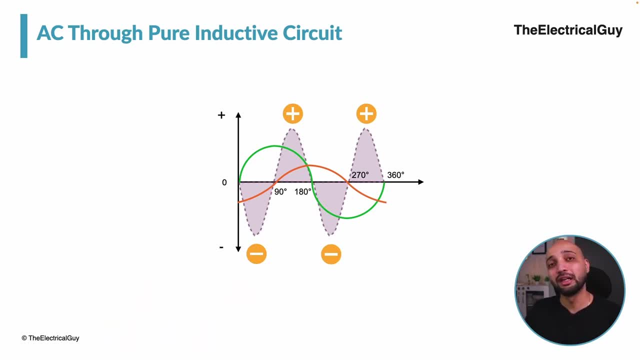 consuming the power from the circuit and negative indicates it is delivering power back in the circuit. now this is exactly opposite than what we have saw in the resistive circuit. resistive circuit, we have saw you calculate instantaneous power at any instance of the waveform. the resultant power is always a positive power and that we call it as active power. but in case of 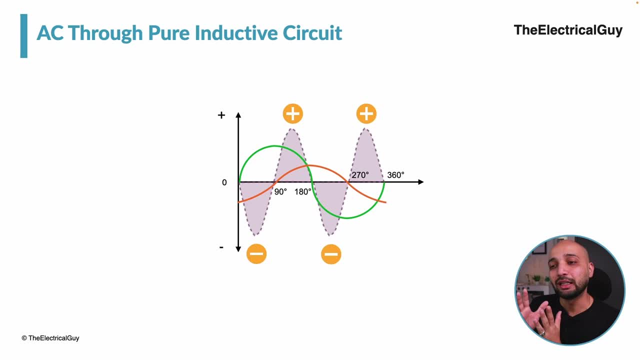 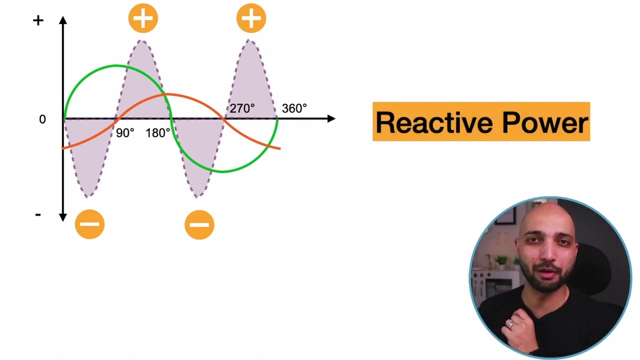 inductor. that is not the case, you will see. the power is zero because the positive peaks and negative peaks are canceling out each other, so the resultant power is zero. and whenever power goes negative, we call that power as reactive power or imaginary power. right, clear, so actually inductor. 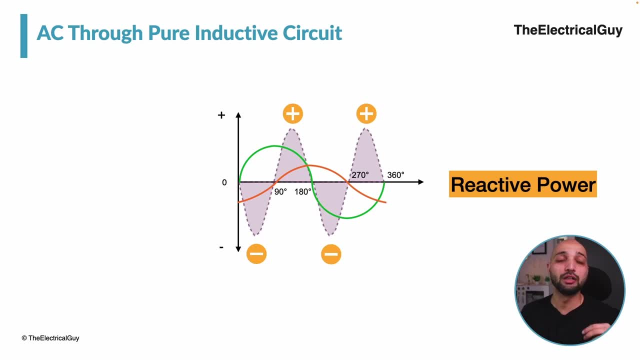 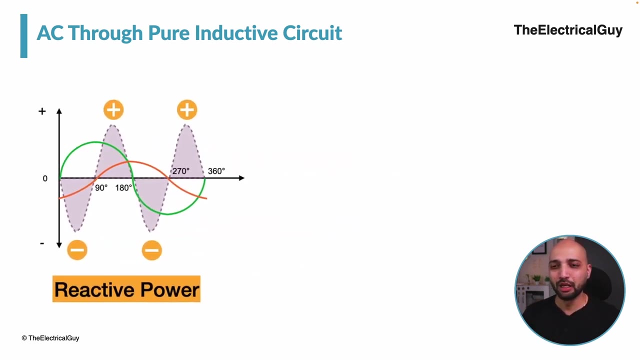 is not taking any actual power to- you know, do perform some useful work. it is taking imaginary power or reactive power. now we can also prove this using the mathematical expression that the inductor do not consume any active power. so let's do that here. so power formula we know is p is equals to: 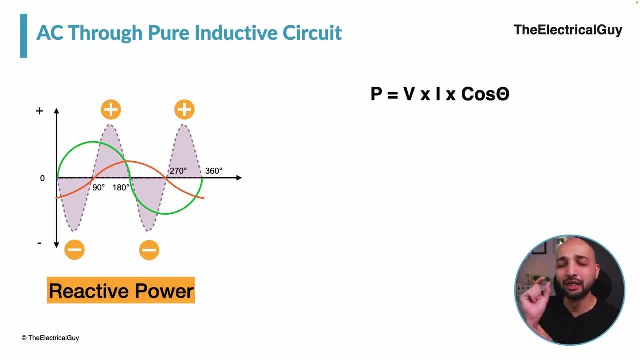 v times, current times, the cos theta. now, what is theta? theta is the angle between voltage and current. now, in case of resistive circuit, that was zero and hence the power was simply p is equals to v times current clear. but in inductive circuit, the theta, that is the angle between voltage and 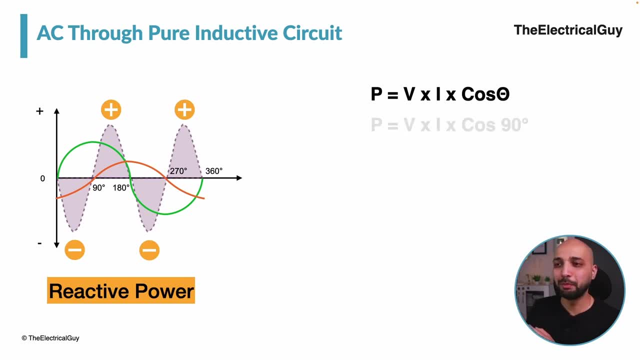 current is 90 degree, so it will be. p is equals to v times, current times, cos, cos 90 degree. and if you find the value of cos 90 degree, it is zero, right? so the resultant power is zero watts. now we are talking about actual power. 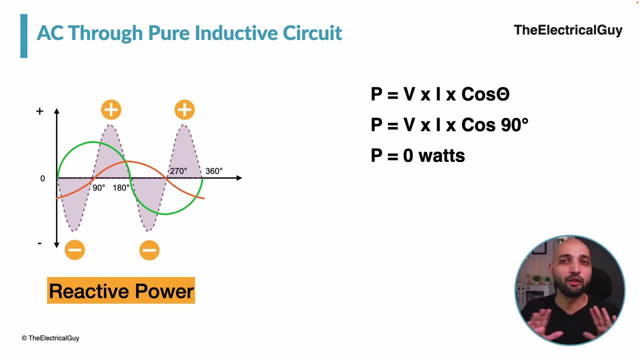 so whenever there is a purely inductive circuit, it will not consume any actual power, right? but since we are talking here both about voltage and current, the consideration of cos theta may not be the right choice. so what we have to do is we have to consider sine theta. so if you put theta value 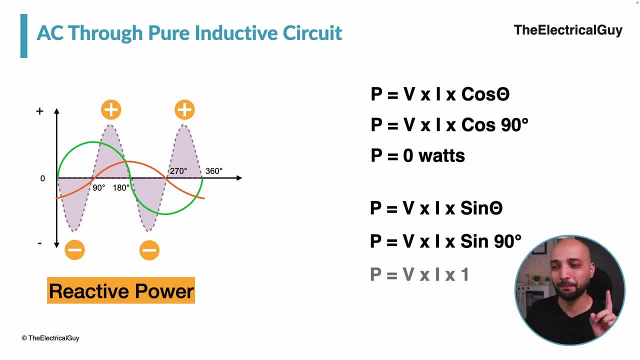 in this equation, that is sine 90 degree and that is one. so the resultant power that you will get is: p is equals to v times current, and that is var. the unit is var, Dat is volt ampere reactive, and this is reactive power, this is imaginary power. 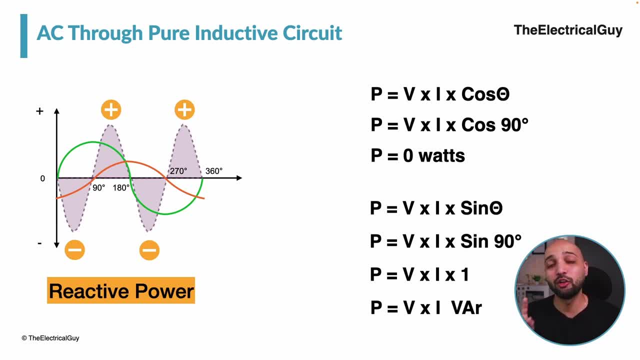 this is not actual power and since this is the reactive power, we do not denote it with letter p. it is denoted by letter q. always remember that and do not get confused between watts and var. watts is where there is only active power and we use var volt. ampere. reactive or kvar. kilo volt. 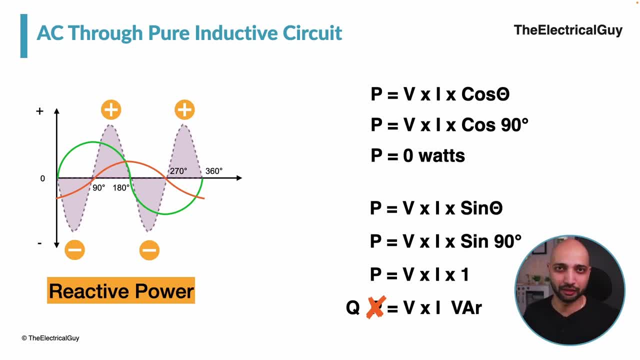 ampere reactive whenever there is a power present in the circuit. so since inductor is consuming reactive power, the unit is var right, and that is the situation of power in an inductive circuit. very, very interesting thing to understand. now let us quickly summarize the video we will discuss about what we have discussed. 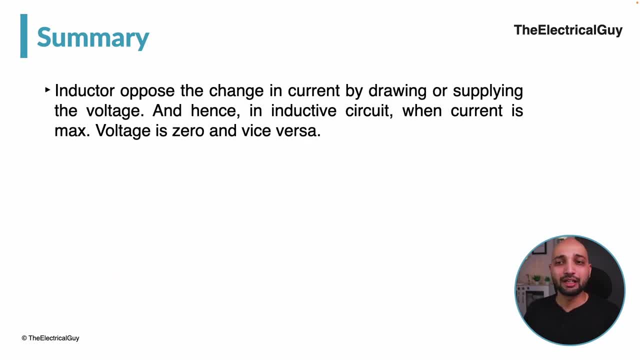 so far in the quick summary part here. inductor opposes the change in current by drawing or supplying the voltage, and hence in inductive circuit, when current is maximum, voltage is zero and vice versa. in inductive circuit current and voltage are out of phase by 90 degree purely.